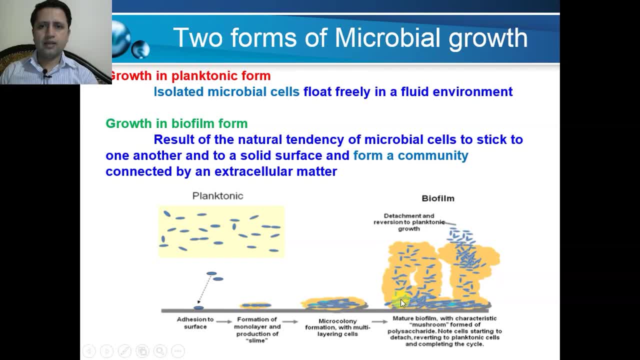 planktonic form of microbial cells. Here you can see examples of planktonic cells which are freely available, which are freely moving into the fluid environment. And then another one is the growth in the biofilm, form and result of the natural tendency of the microbial 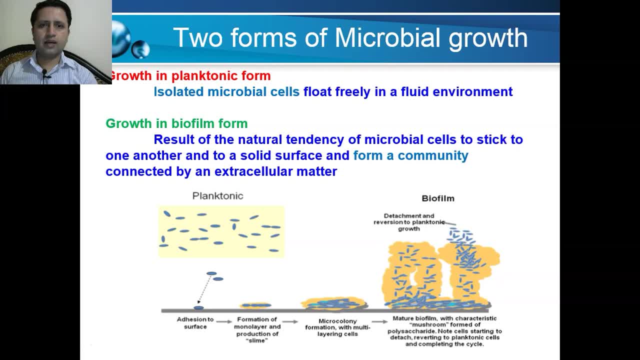 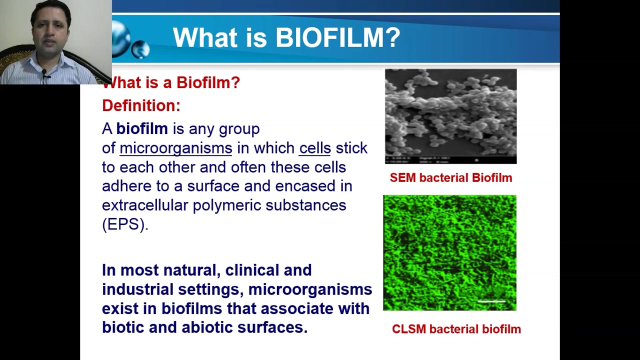 cells to stick one another into a solid surface and form a community which is connected by an extracellular matter, And this is called biofilm. Here you can see this is the structure of a biofilm cell which are formed on the surface. So what is actually a biofilm? A biofilm is actually. 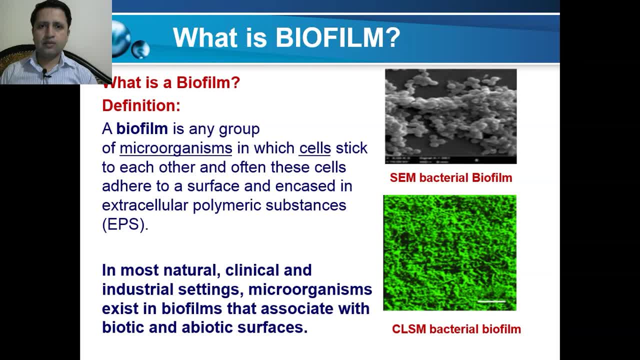 any group of microorganisms in which cells stick to each other, and often these cells adhere to a surface and encase in an extracellular polymeric substances. So what are extracellular polymeric substances? Extracellular polymeric substances are the cells which are formed on the surface. 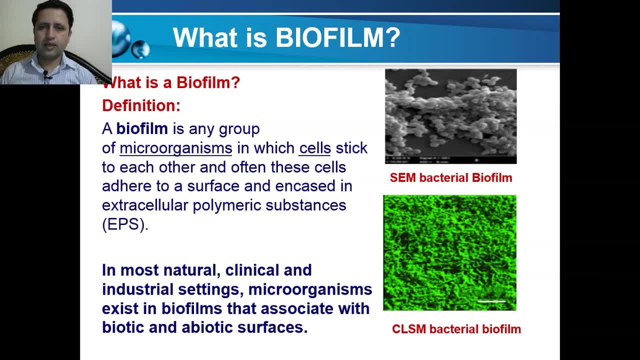 which are produced by bacterial cells extracellularly, And these extracellular polymeric substances are protein, polysaccharides, eDNA and some lipid in minute quantity also, And extracellular polymeric substances helps in the attachment of bacterial cells and bacterial cells are. 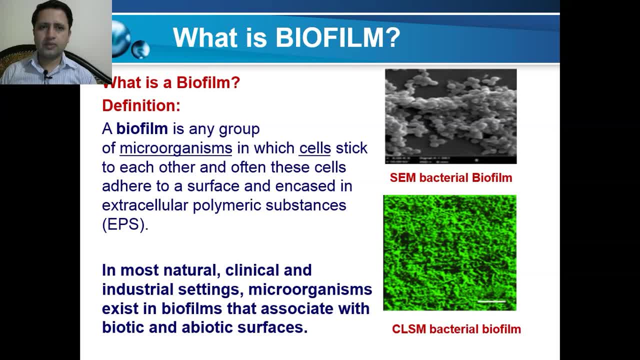 embedded in this extracellular polymeric substances. These are two structures of microbial biofilm. This is the same scanning electron microscopy image of bacterial biofilm And this one is the confocal laser scanning microscope after staining of the bacterial biofilm. So in most natural clinical and 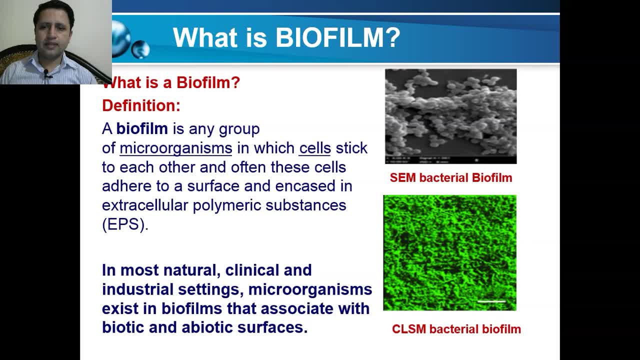 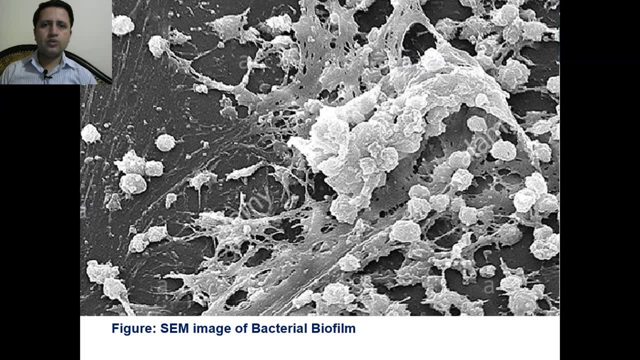 industrial settings. microorganisms exist in biofilms that associate with biotic and abiotic surfaces. Here you can see in large same image of a biofilm And this is the same scanning electron microscope. after staining of the bacterial biofilm. you can see many bacterial cells are embedded. 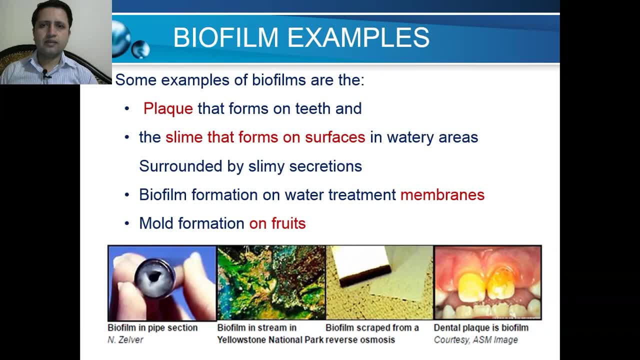 into the EPS. Here are some examples of microbial biofilm. One of the example is the dental plaque. In this diagram you can see dental plaque biofilm formation on the teeth's surface and the slime that forms on the surface in the watery surface, which is algal green biofilm. 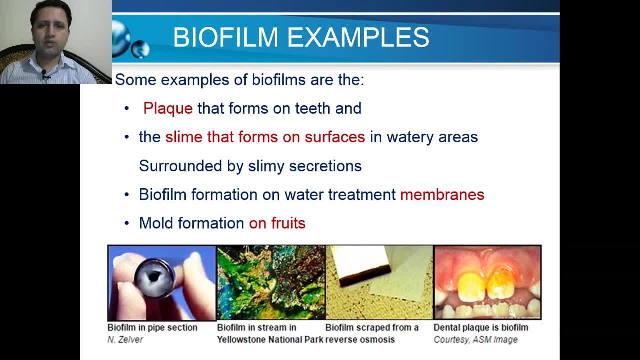 secretions and biofilm formation also occur on the treatment membranes which are used for the filtration of different wastewater, and you can also find mold formation on different foods and you can see the rhizopus formation on the bread and many examples like biofilm formation in the water pipe section also. Here you 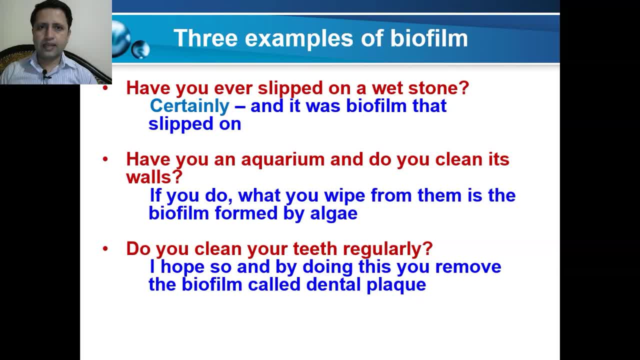 can see some other examples, like: have you ever slept on a redstone? Certainly, and it was biofilm that you slept on- and have you an aquarium and do you clean its walls? and if you do so, what you wipe from them is the biofilm formed by the 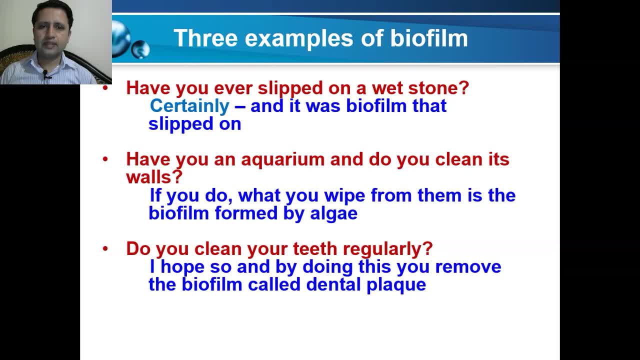 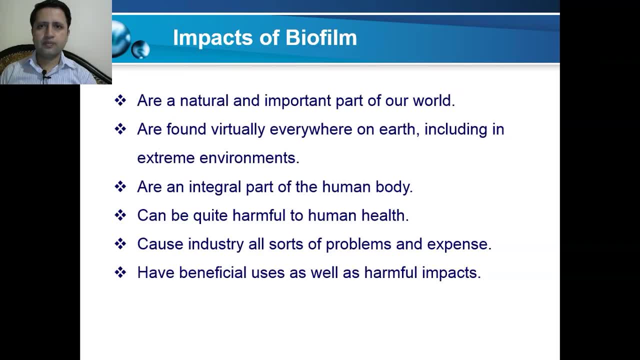 algae and also, do you clean your teeth regularly? I hope so, and by doing this, you remove the biofilm called dental plaque, biofilm. Here are some impacts of. biofilm are a natural and important part of our society and it is found virtually everywhere on the earth, including extreme environments. 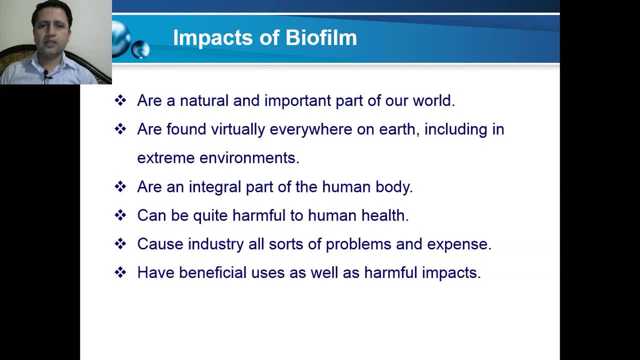 also, and they are integral part of the human body. it can be quite harmful to human health and it can cause industry all sorts of problems and expenses, like food spoilage, contamination of equipment, contamination of food material. and it helped beneficial uses as well as harmful impacts. like it can be used for bioremediation purposes. 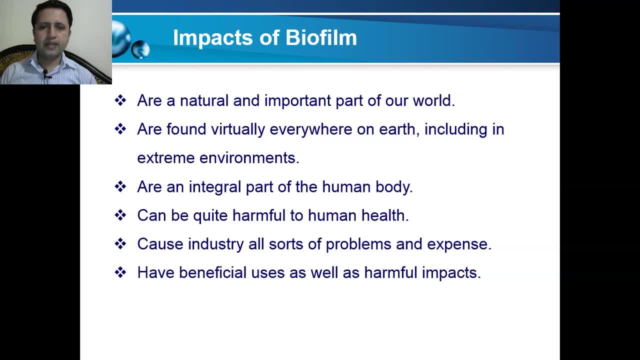 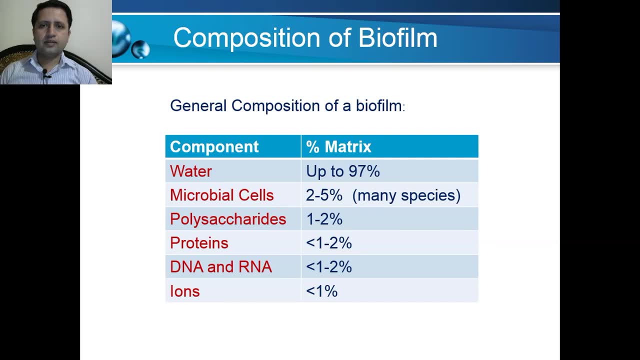 It can be used for bioenergy production. Many enzymes can produce using microbial biofilms. also In this slide we can see composition of biofilm. Here is the general composition of biofilm. water is present up to 97% in the microbial biofilm and microbial cells are present from two to five percent. 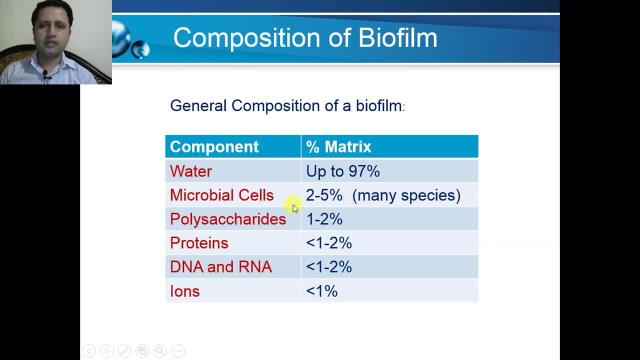 It can be single species and it can be many species also. Then polysaccharide is present one to two percent. protein is present less than one to two percent. DNA and RNA are present one to two percent, and small quantity of ions are also present in the microbial biofilm. 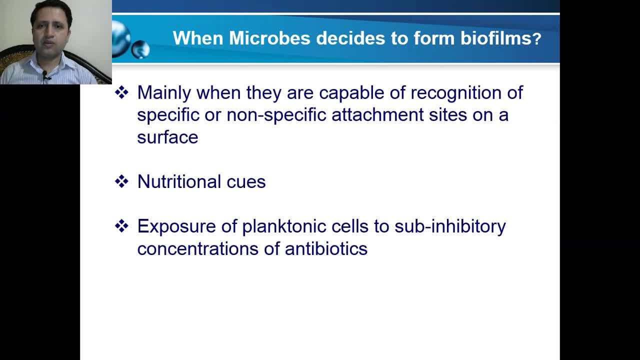 And when microbes decide to form biofilm, or why microbes decide to form biofilm? there are many reasons. Some of the reasons are presented here. mainly when they are capable of recognition of specific or non-specific attachment sites on a surface, They like to form biofilm because bacteria love to live in the form of biofilm and there 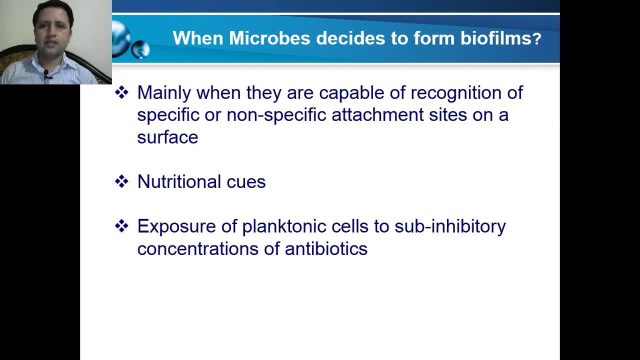 are nutritional cues also And there are many limitations Due to which bacteria biofilm. bacteria like to form biofilm whenever there is a limitation of nutrients. there are limited nutrients available, So bacteria like to form biofilms. And then exposure of the planktonic cells to the sub-inhibitory concentration of antibiotics. 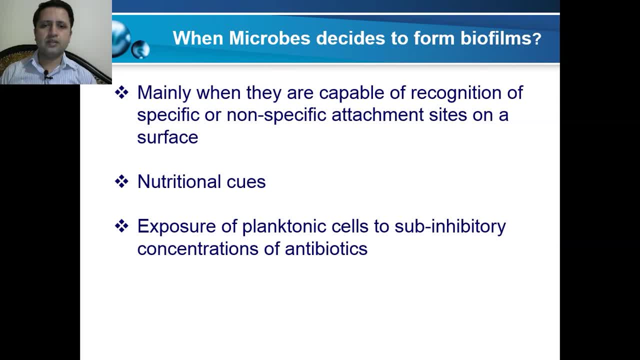 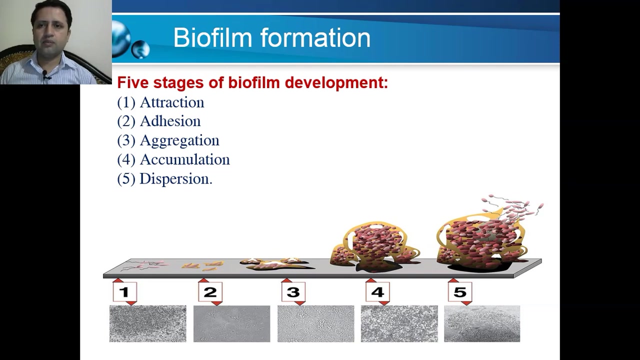 that when you add sub-inhibitory concentration or when you give sub-inhibitory concentrations of antibiotics to the patient, So then there is a chance that bacterial cells start forming biofilm and eventually they are resistant to the antibiotics. Here you can see biofilm formation. 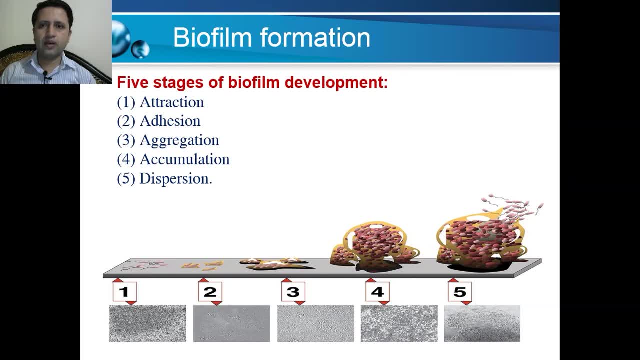 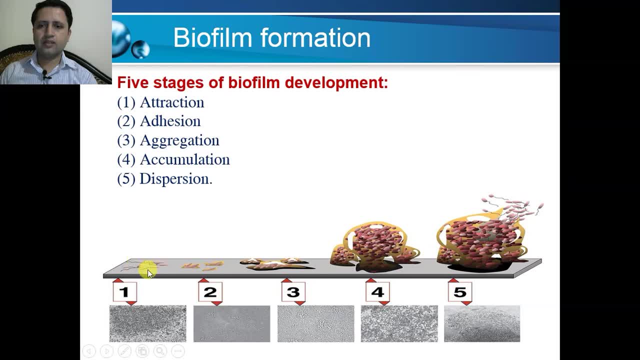 The first stage is that: the biofilm. The first stage is that: the biofilm. The first stage is that the microbial cells attract on the surface and then they like to adhere. their adhesion occur on the surface and then aggregation occurs. Biofilm: bacterial cells from different colonies and they aggregate themselves on the surface. 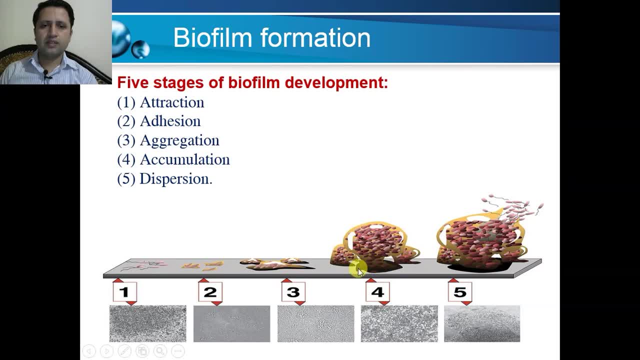 and then mature biofilm formation occurs. Bacteria produce some extracellular polymeric substances and they encased their cells into the EPS, which is aliazis—aia Aiazis in the epa protective layer. eps is the extra singular polymeric substances and bacteria in case 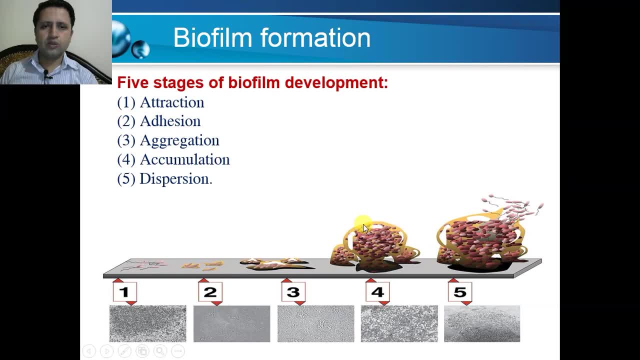 and protect their self in this eps. so whenever you add antibiotics or chemicals, so it is very difficult for bacterial cells to penetrate the eps, which is a gel like structure, and after uh maturation, after maturation of the biofilm, the biofilm also start to disperse some of the 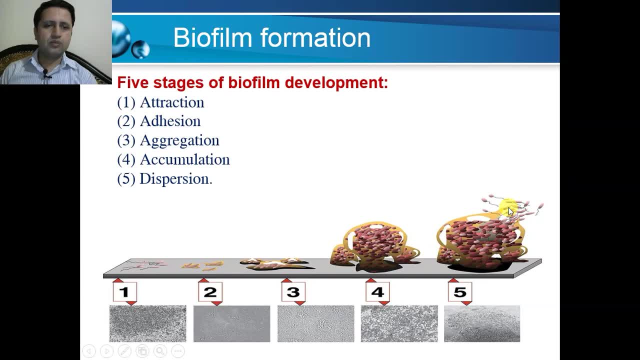 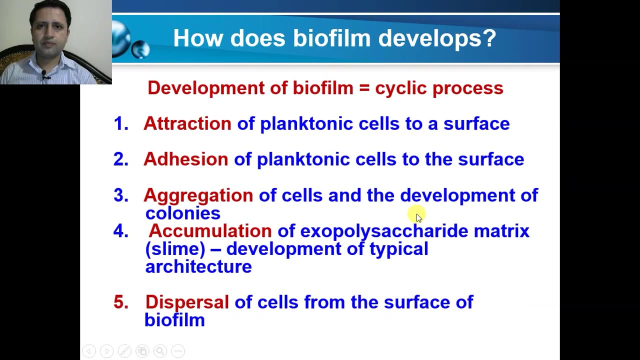 bacterial cells are dispersed from the microbial biofilm and then they start attaching on the other surfaces, which are the empty surfaces, and then they again start the biofilm formation cycle. here you can see the explanation of the biofilm development. in the first step, attraction of planktonic cells to the surface. the second: 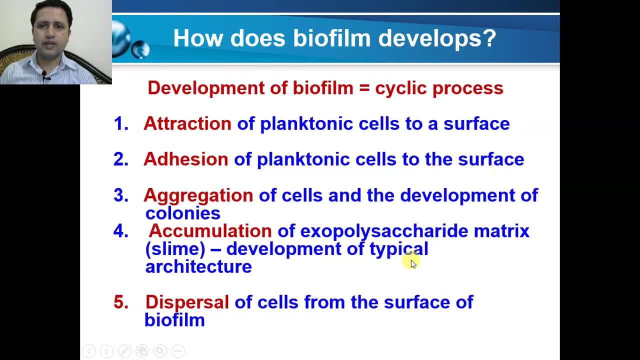 stage is the adhesion of planktonic cells to the surface and then aggregation of cells and the development of colonies occur. and in the fourth stage, accumulation of the exo polymeric substances, which is, extracellular polymeric substances, which are also called as a slime, and the development of. 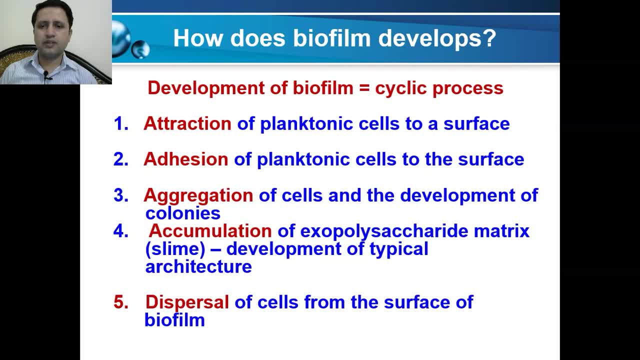 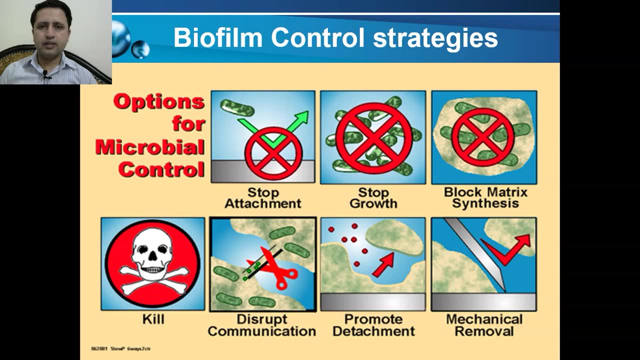 the fifth stage is the dispersal of cells from the surface of the biofilm occur and this biofilm cycle again start from the attraction and then addition, aggregation, accumulation and dispersal. there are different strategies which can be used for the biofilm control. here are some briefly. 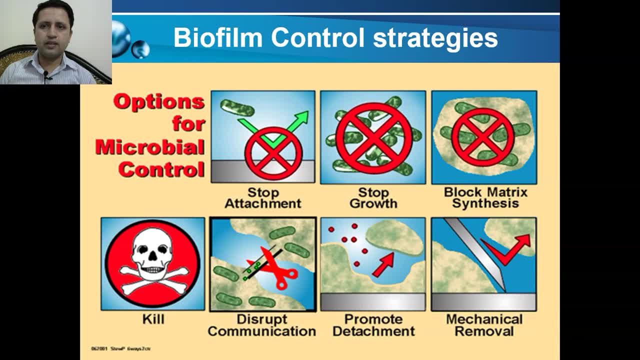 discussed the strategy briefly showed these strategies here that you can graphs describe how biofilm may flow within the body. we serve the biotaあと a wide range of payoff activities different ways. biospec, zukang, run the putting additional own. you give some antibiotics etc. to stop the growth of microbial cells. are to 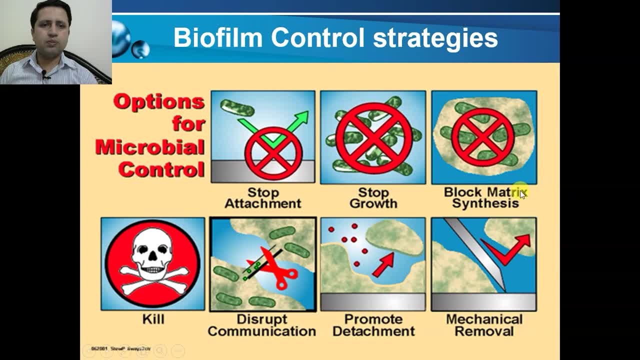 kill the microbial cells. and the third strategy is to block the matrix synthesis. matrix synthesis is the production of the extracellular polymeric substances. you can also stop this. extracellular polymeric substance is production and one of the strategy is to kill the bacterial cells. so one of 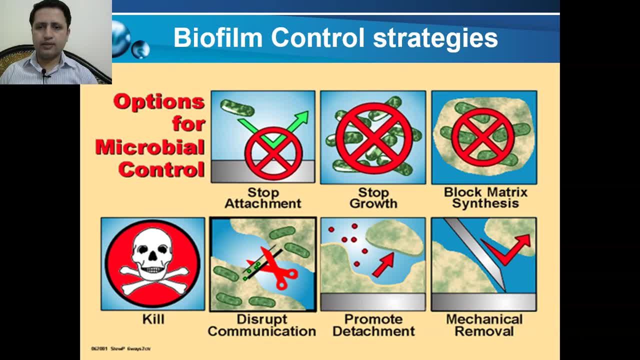 the strategy is to kill the bacterial cells. so you can use chlorination and you can use antibiotics, or you can use plant products to kill the bacterial cells. and here another strategy is to disrupt the communication. you can also disrupt the communication by by targeting the signaling molecules, which 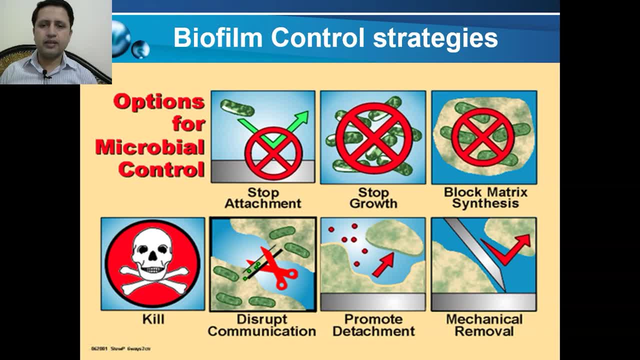 is called language between the bacterial cells in which they produce some signaling molecules like they want to form by film formation. so they produce some signaling molecules and then bacterial cells sense these signaling molecules and their genes are activated and then they produce some molecules for the biofilm formation. so we can also disrupt this communication by different. 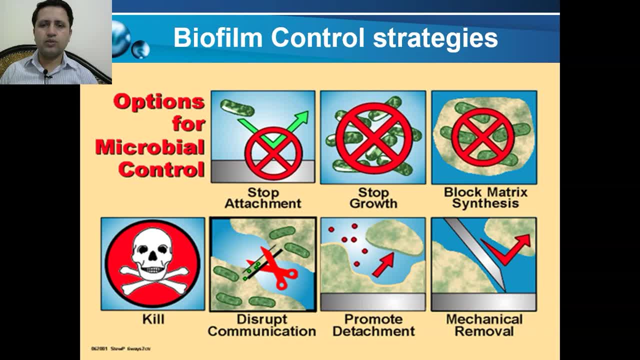 ways: by using some plant-based compound, by using synthetic compounds, and also we can to do quorum quenching, to quench the bacterial cells. we can also control the biofilm formation by promoting the detachment. once biofilm is already there, we can use some chemicals to detach the biofilm, to disperse the biofilm. another: 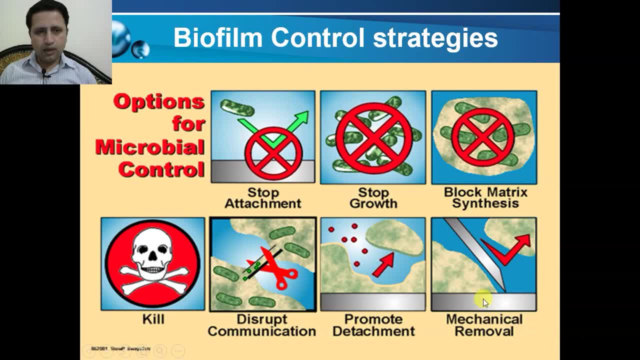 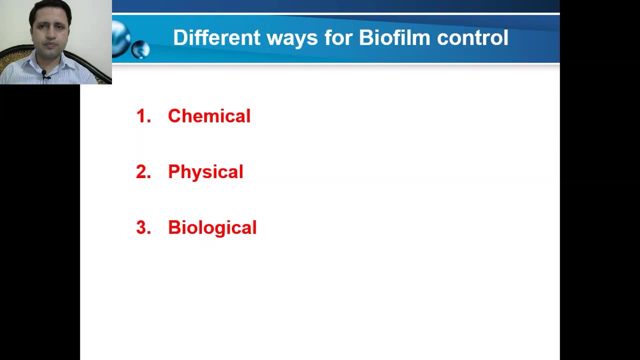 strategy is the mechanical removal. we can also mechanically remove the biofilm by using some physical tools like by knives, by scrapers etc. to physically remove the biofilm from any surface. so there are different strategies can be used for the biofilm control: chemical treatment, physical treatment and biological treatment in chemical. in water treatment we can use 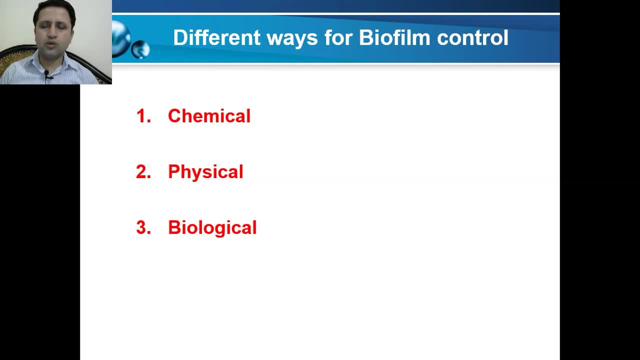 chlorination and in for the human. we can use antimicrobial, another one we can use for the use of radioactivity and other antibiotics, synthetic antibiotics, and we can use some for the physical treatment. we can do some shaking to disperse the attached bacterial biofilm and we can 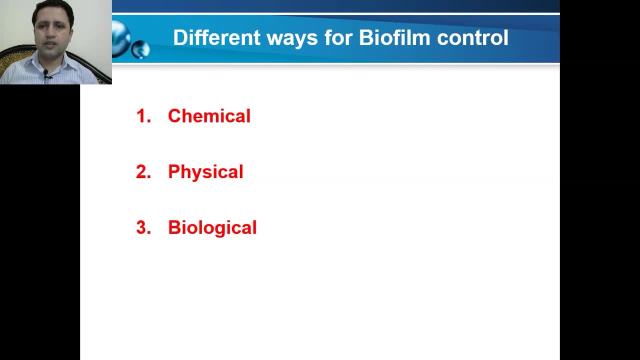 use the scrapers to physically remove the biofilm formation. and we can also do by biological mean. by biological mean we can use some plant-based products. we can use biological base products, like from microbes. we can use bio-detergents, we can use enzymes, etc. to biologically remove, to biologically control the. 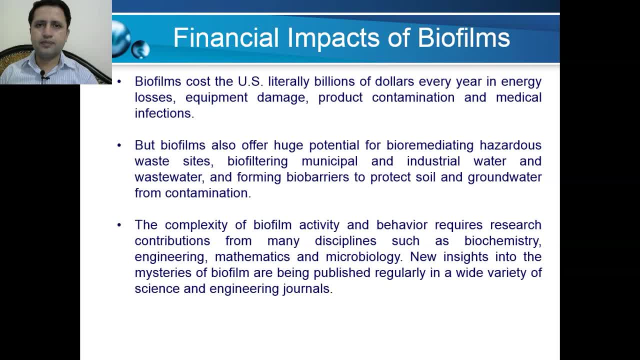 formation of biofilms. there are financial impacts of biofilms, and biofilms cost the us literally billions of dollar area in energy losses in equipment damage, product contamination and medical infections as well. but biofilm also offer huge potential for by mediating hazardous waste sites. 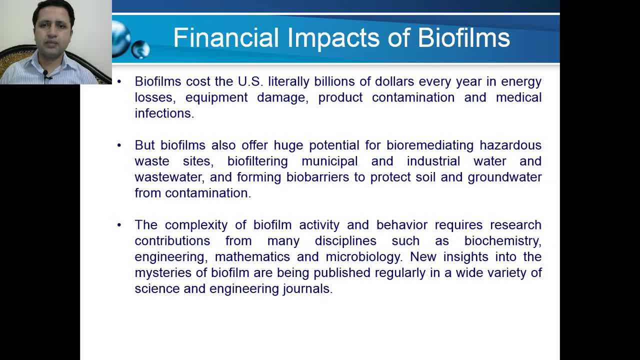 and we can use it for the municipal wastewater treatment and we can even use it for the bio composting, for bio energy production also, and it can be used forming farming bio barriers to protect the soil and groundwater from the contamination also. so there is good side also and bad side also in the 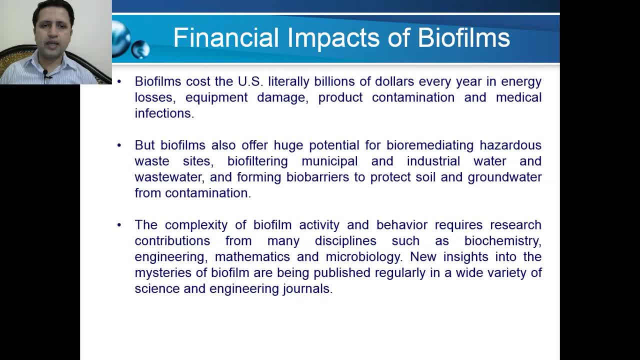 complexity of biofilm activity and behavior requires research contributions from many disciplines, such as biochemistry, engineering, mathematics and microbiology, and new insights into the mysteries of biofilm are being published regularly in a wide variety of science and engineering journals. so I till now, we see that there are two sides of biofilm. one is the good side and 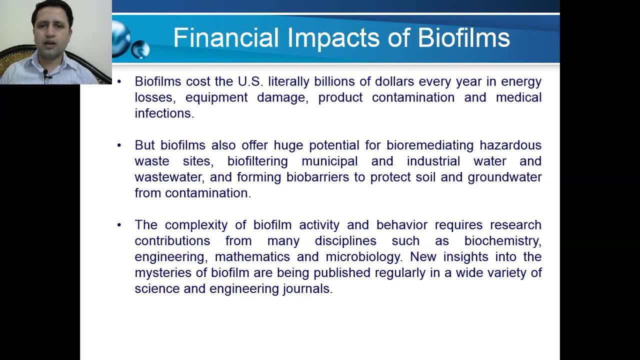 another side is the bad biofilm. good biofilms are also called productive biofilms, which can be used for energy production, which can be used for enzymes production, which can be used for by remediation, etc. and bad, bad biofilm, causing different problems and challenge. they pose different challenges also. 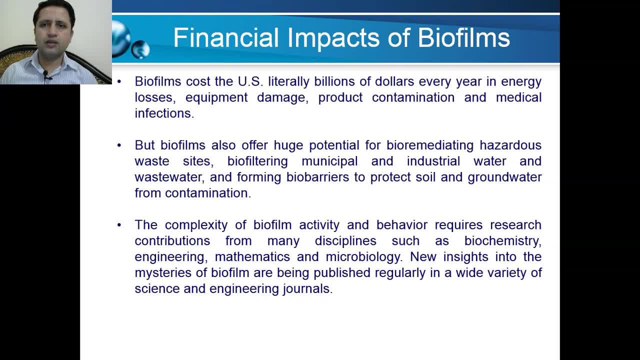 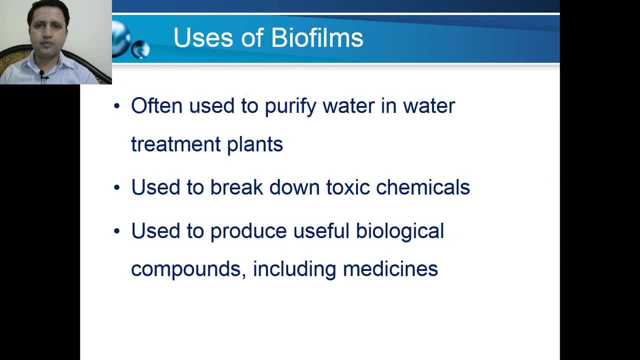 and they cause billion dollars to the different countries and equipment damage, product contamination, medical infections, etc. there are some uses of biofilm. biofilm often used to purify water in the water treatment plants and it can be used to break down different toxic material by by remediation and 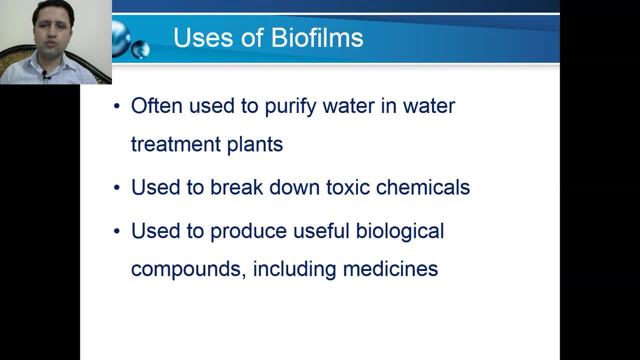 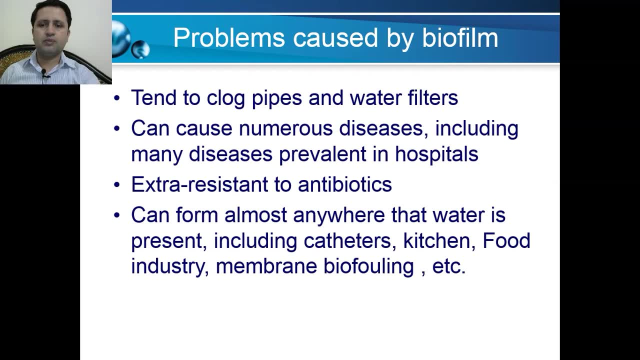 biodegradation and it can be used to produce useful biological compounds, including medicines that can be used to treat diseases and also can be used to treat diseases etc. and there are many problems which can be caused by the biofilm. there are different problems which are caused by biofilm and it can